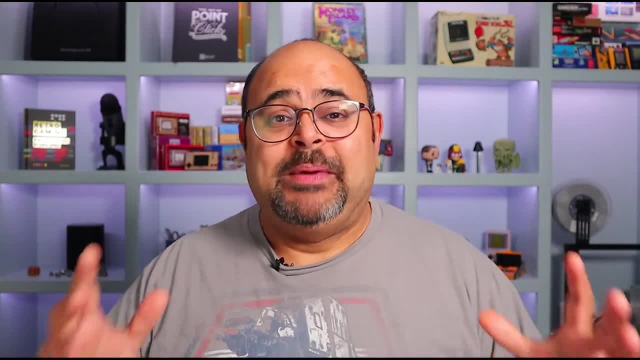 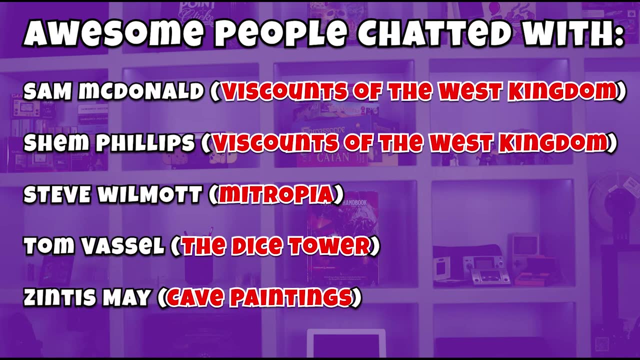 I've got to say from the get-go that I'm not an expert here, but I have spent the last year and a bit interviewing people who have actually been there and done it- proper game designers- As well as doing a whole bunch of research on forums and reading books, And the more I've read 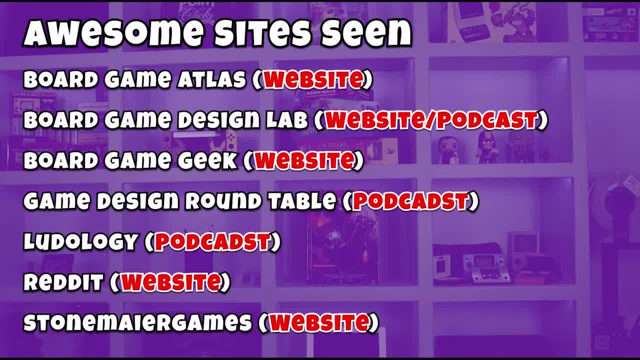 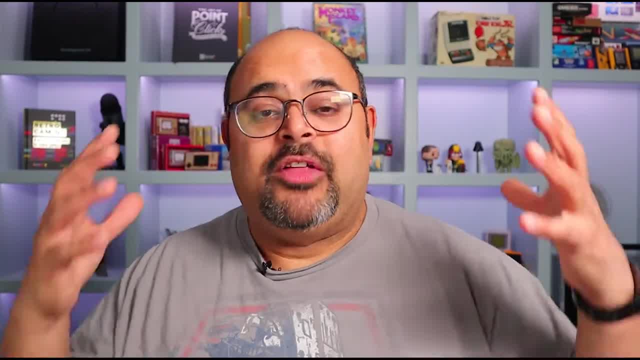 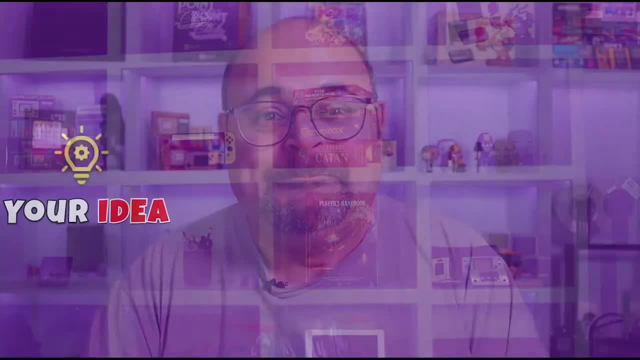 the more passionate and excited I've become about the whole area of board game design. Now, today, like I said, I'm going to be starting off this year with a very quick summary of what it takes to make a board game, And we're going to start with the idea. Game ideas consist of: 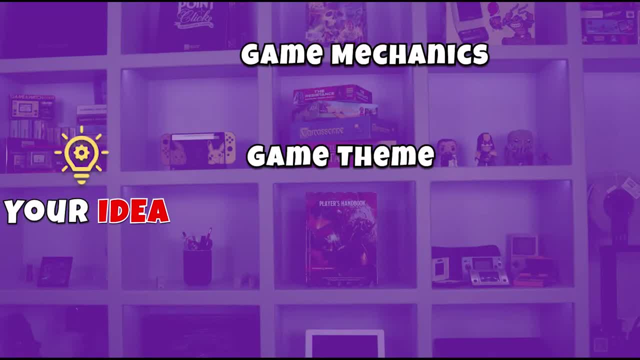 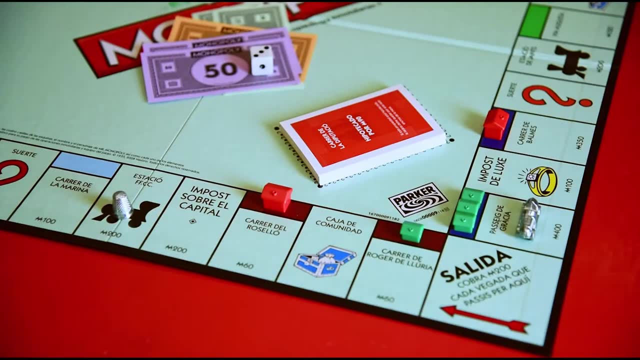 three constructs, and that is mechanics, theme and player experience. Mechanics is how your game works. If you pick up some dice and roll them to move a piece, well, that's a roll and move mechanic. If you pick up cards or draw cards from a pile, 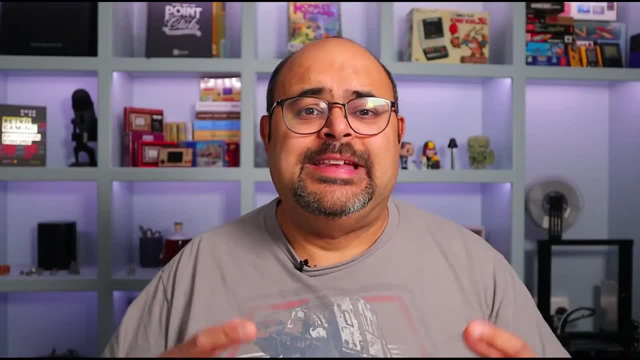 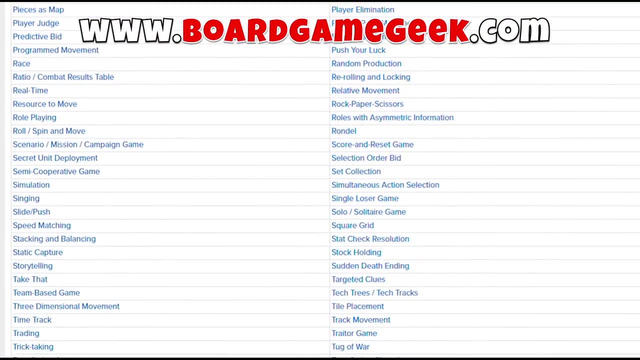 that's a draw mechanic. If you use those cards to build a deck, then that's a deck building mechanic. In fact, there are over 250 plus documented mechanics on Board Game. Geek Mechanics together form the engine of your game Theme. on the other hand, 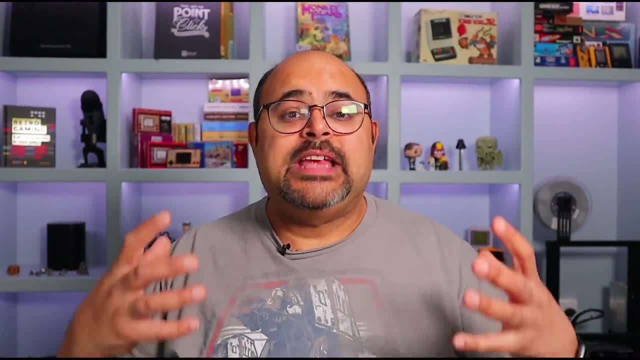 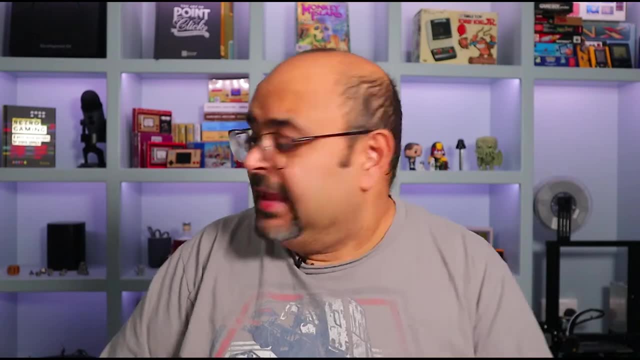 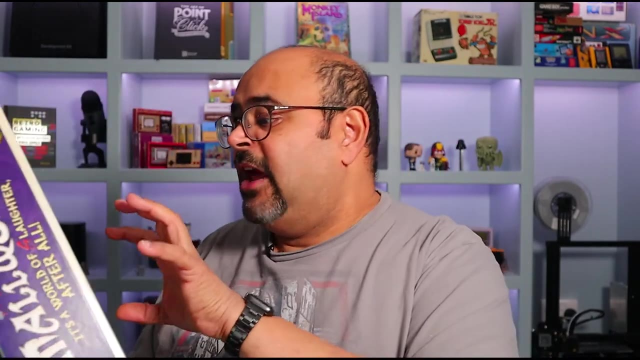 is the context around those mechanics. It creates a immersive environment for your players to exist. It helps them stay engaged in the game. A game like Small World, which is a perfectly fantastic game, I think, can be enhanced by a compelling theme like the World of Warcraft. 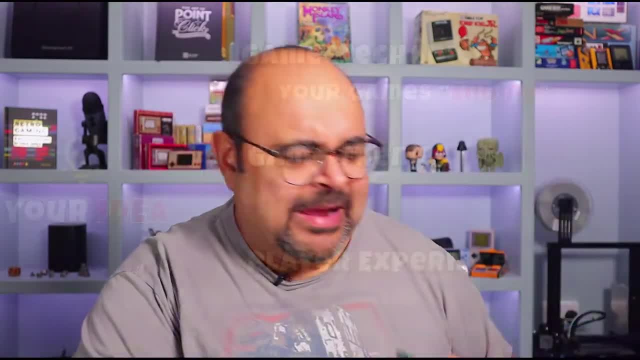 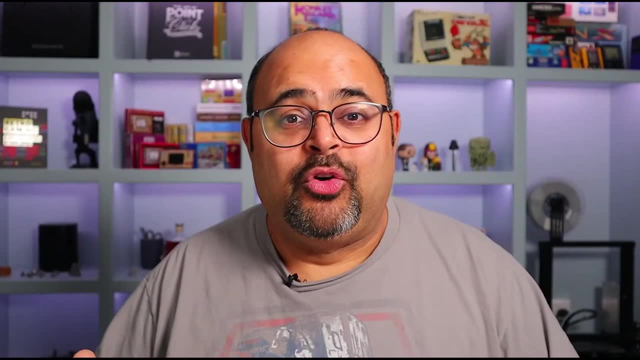 I think this is gonna be an excellent game when I finally get around to playing it. Theme creates that engagement that you want from your players, And the third part of your idea should be the player experience. What do you want your players to feel? 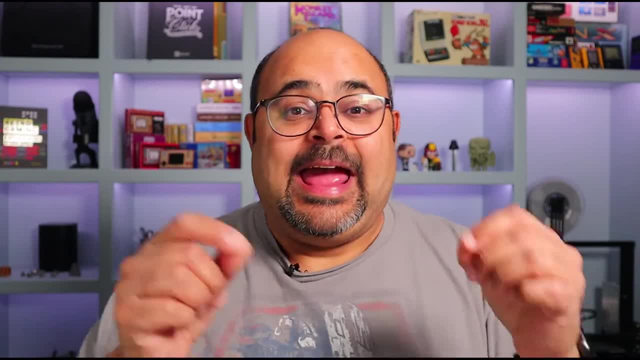 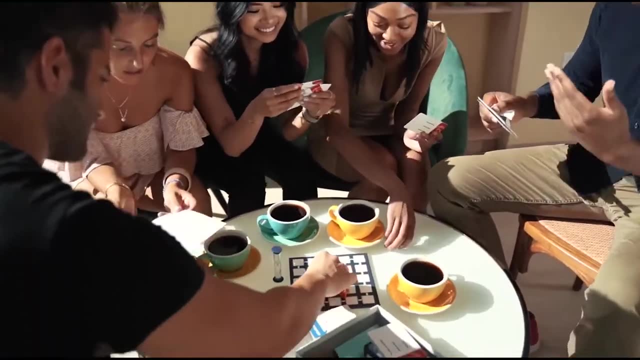 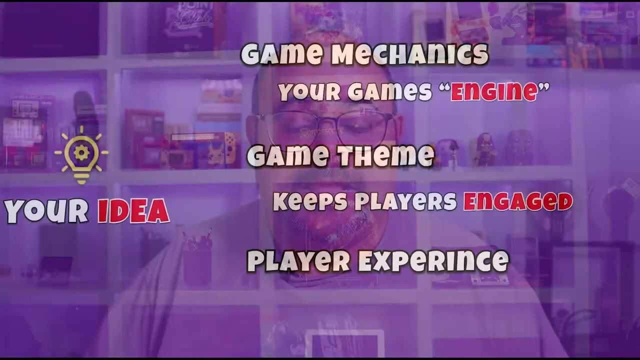 And in fact, this is the thing that will keep players playing it and replaying it over and over again. Do you want your players to feel a sense of tension or is it an easygoing party game? Do you want clever thought and strategy or do you want lots of free-flowing conversation and laughter? 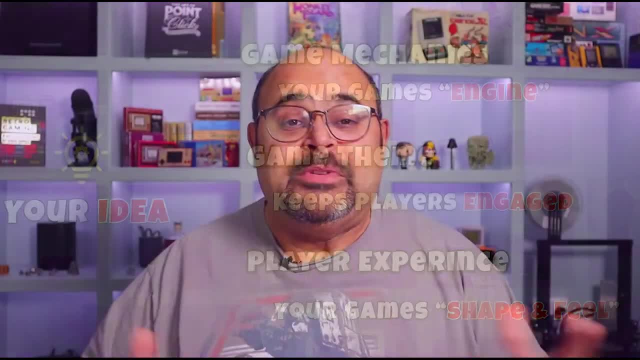 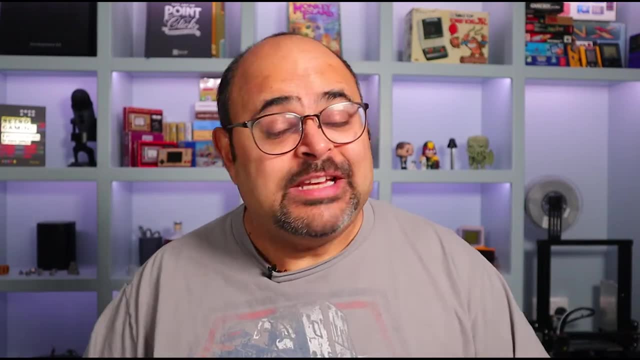 All of this will shape how you develop your game. Now, it's easy for me to say that games need an idea to start with, but where do you get those ideas from? Well, here are six places. you can find some inspiration, starting with number one: playing lots of games. 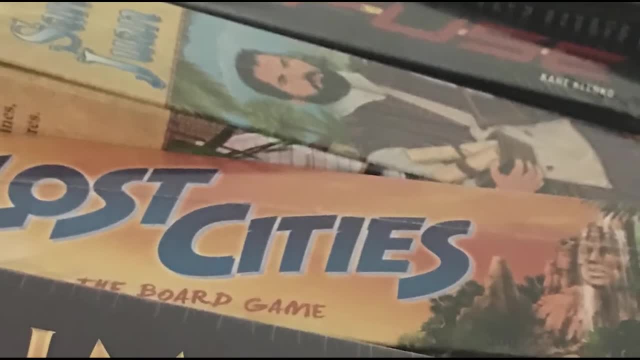 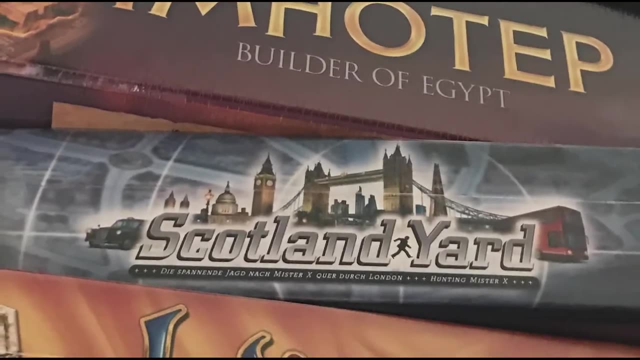 Games have changed dramatically over the last 10 years, And if the last thing you played was Trivial Pursuit or, dare I say it, Monopoly, well, you really need to get out there and explore what else is available, because there's a huge variety. 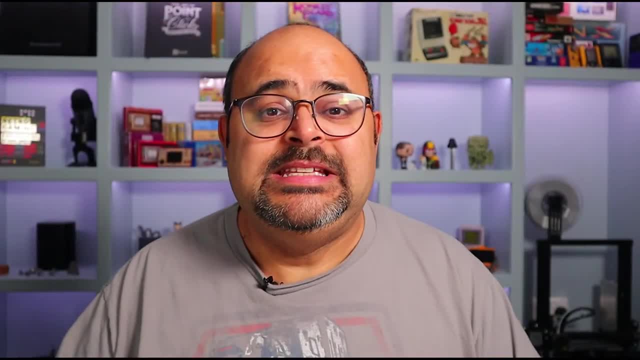 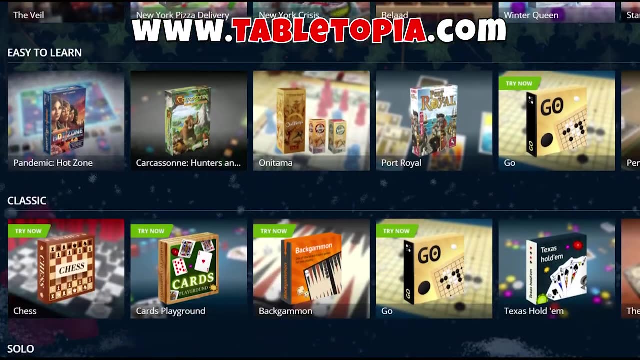 of different kinds of games now, And if you're restricted in actually meeting people to play games because of the lockdown, well that's okay. Services like Tabletopia exist which allow you to go and play a whole range of games online with real-life people. 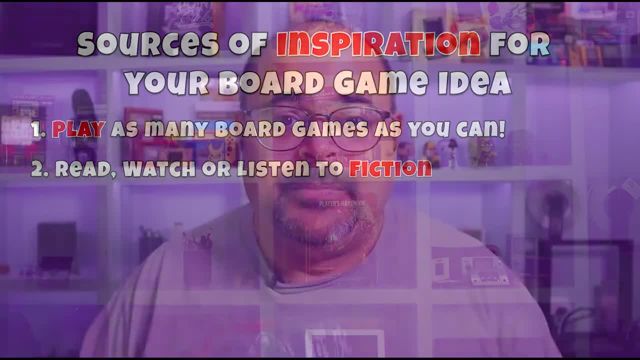 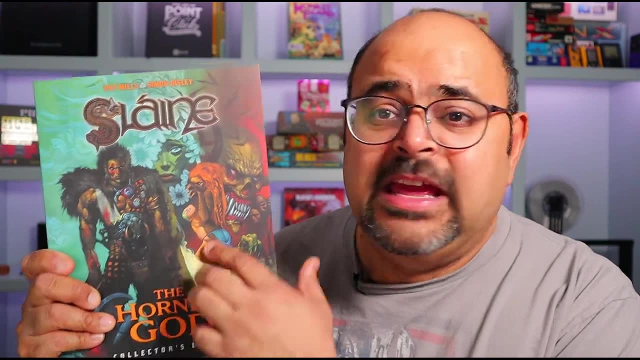 Two: watching or reading or even listening to fiction. I recently got this graphic novel Slain. It's all about a Celtic barbarian from the world of 2000 AD. This would make an amazing world for a board game. Well, what about Mandalorian? 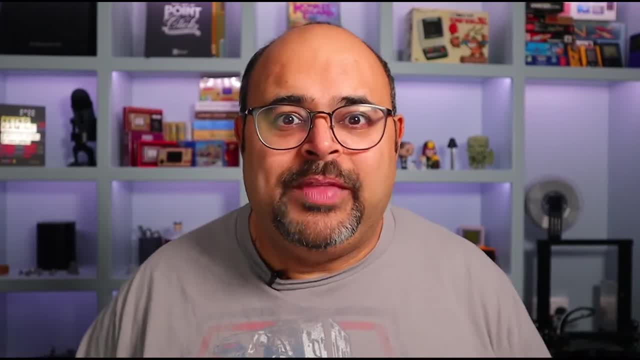 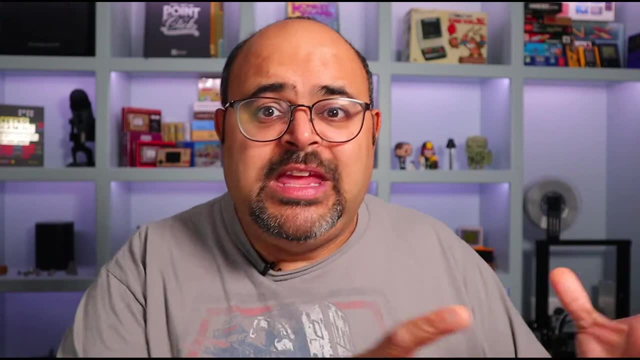 Can you imagine A card game based in that world? How cool would that be? Watching game reviews online is a great way of finding out what's in vogue, what the latest fashion is, both in theme and mechanics. It allows you to see whether your idea 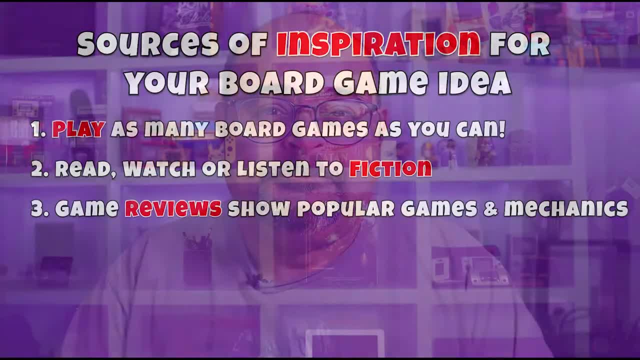 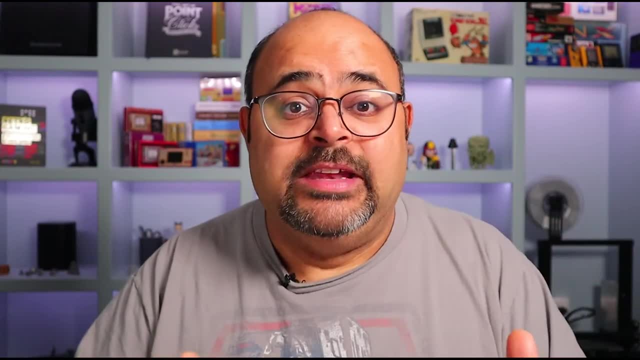 doesn't already exist, Talking of which forums like Reddit or BoardGameGeek or BoardGameAtlas are a great place to go and see whether your idea is in fact valid or whether someone has already beaten you to the post and done something very similar. 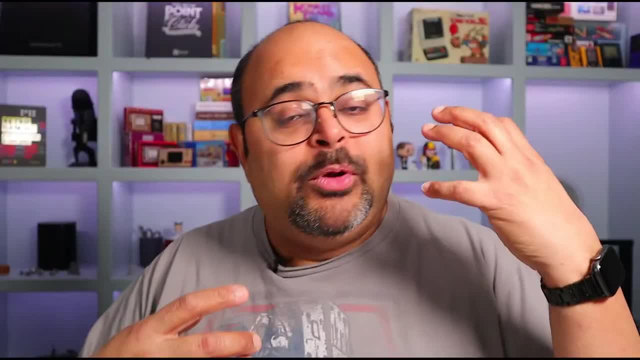 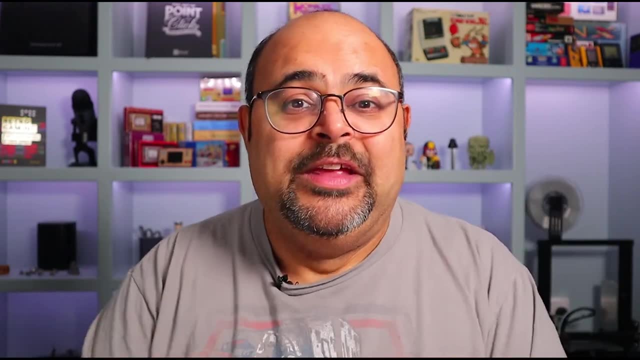 It's a great place, I think, to bounce ideas of other people, other people who have gone through the process. You can ask all kinds of questions and get some really, really useful feedback early on in your development stage. Five: testing other people's games. 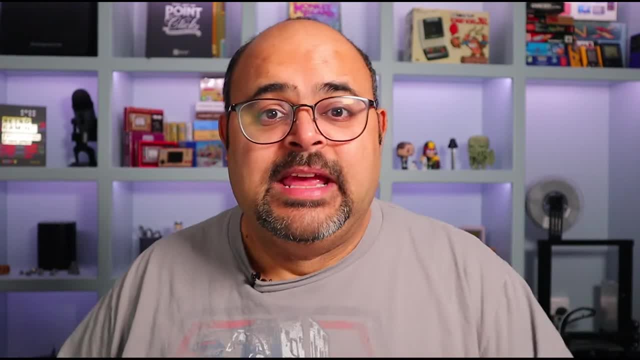 If you're on a forum, you're often gonna come across people who are looking for playtesters- that is, someone who's gonna go out and test a game. Usually, you'll be able to download the instructions and the materials you need. 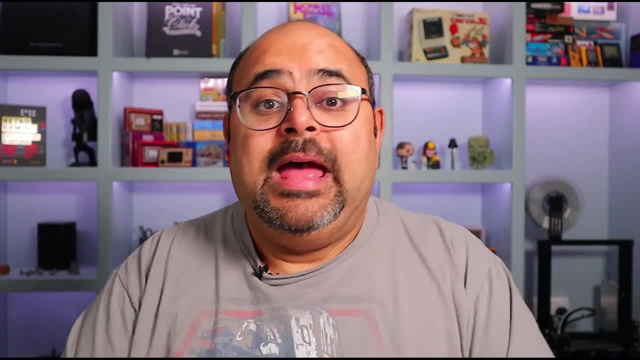 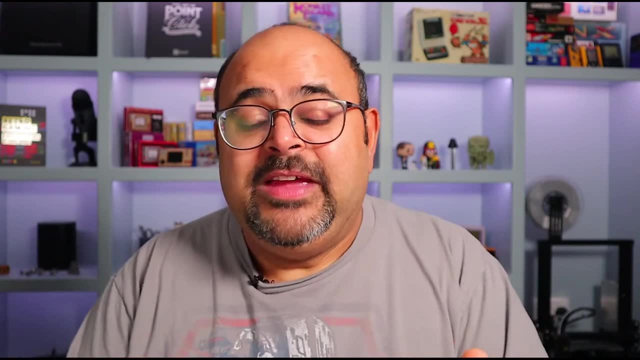 to create your own version of the game and then test it, play it. If you can't do that, then you can pop along the table and that's another place again where you can test other people's games. Now the benefit here is twofold. 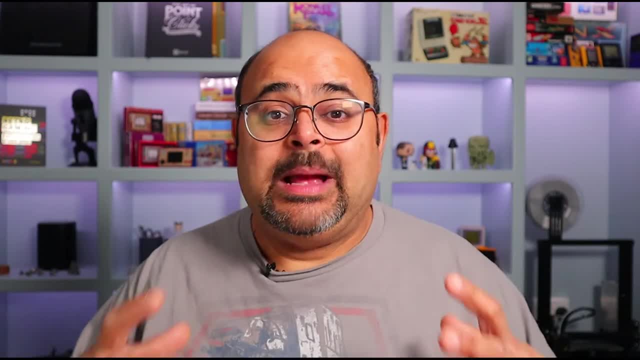 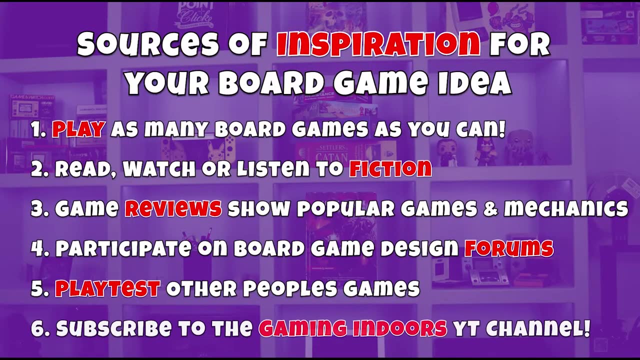 One, you're helping someone else develop their game, but you're also picking up skills in understanding what you should be looking for in a good game. And six is my own channel, Gaming Indoors, a place where you can find- hopefully, 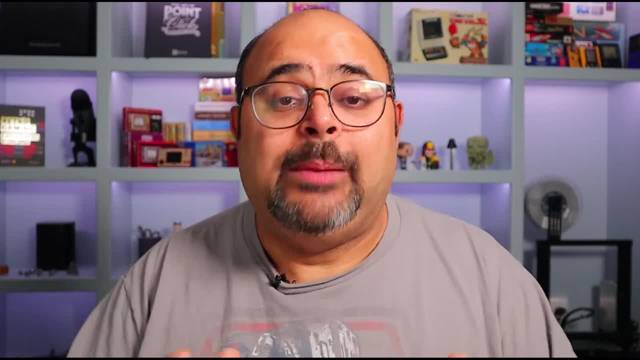 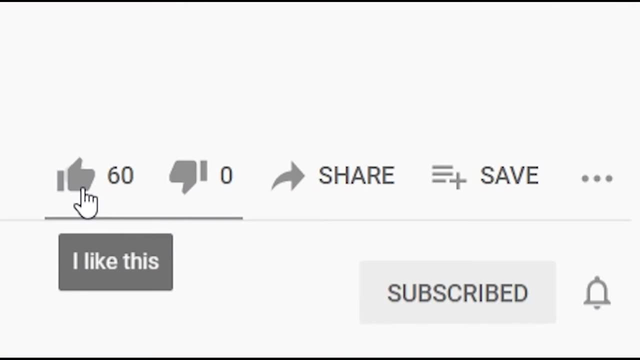 inspiring videos and interviews and little tidbits of information to help you on your game design journey. Hopefully you're finding this video really useful and, if you are, please do click that little thumbs up button because more people will get to see it when you do. 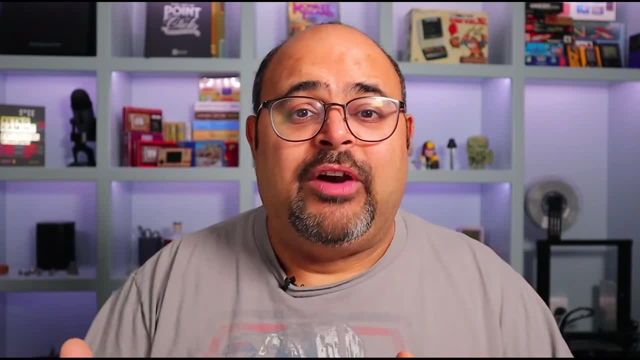 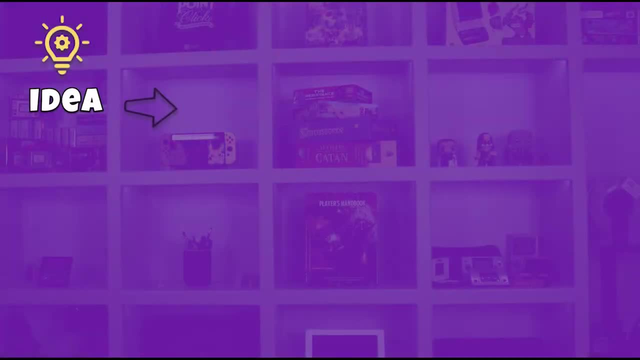 Okay, so we've got our idea, we've got our mechanics, we've got an idea for our theme and we've got some player experience that we want our players to feel. The very next step is to take that and make something tangible, make a prototype. 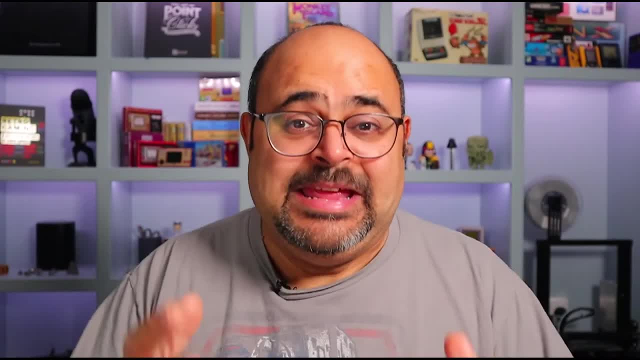 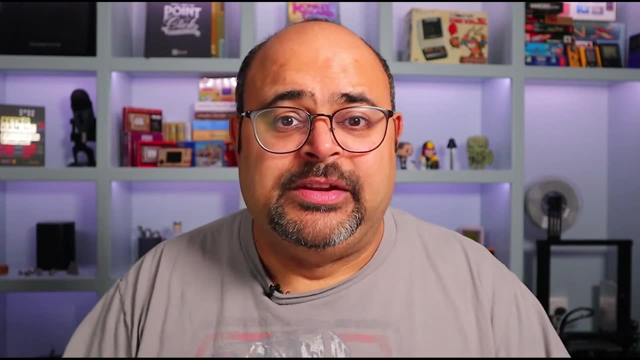 Now the prototype is the first in very many versions of your game. You're gonna do this a lot, so you don't wanna spend too much effort or time in building it. In fact, really, what this whole step is about is identifying the components you're gonna need. 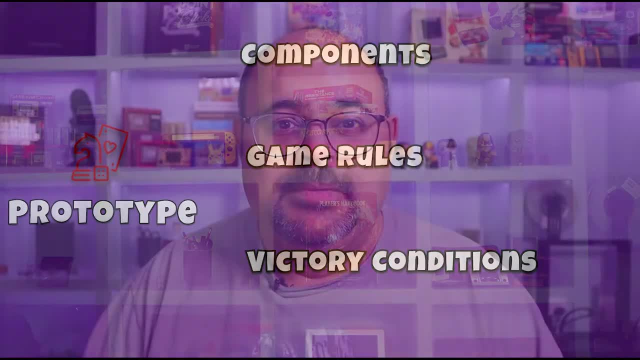 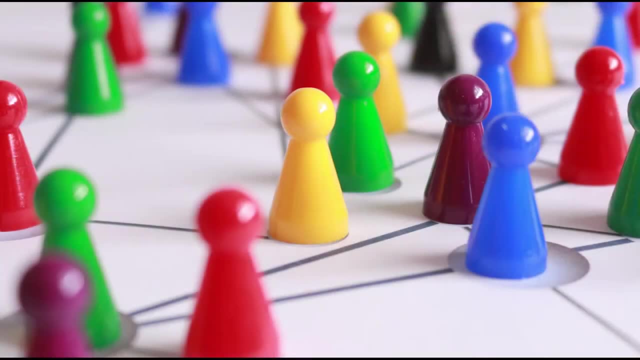 and then applying rules and victory conditions to that. Now, when it comes to components, I don't just mean playing pieces, I mean the playing area as well. Are you gonna use a board, for example, or is this just gonna be a card game? 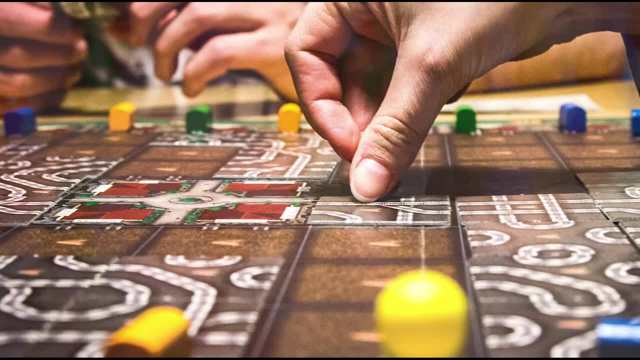 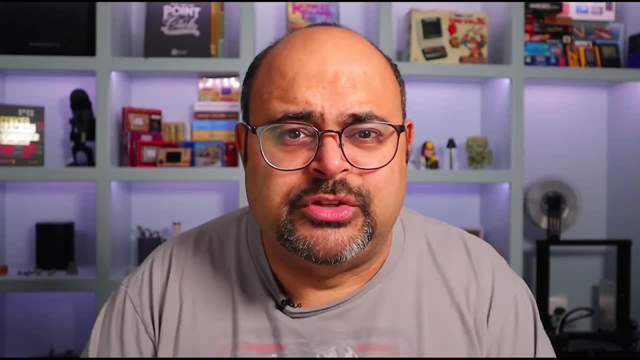 If you think in the future you might want to publish this game, you wanna make sure those components and playing pieces and the playing board aren't too complex, that they're scalable and affordable when mass-produced. Okay, so looking for some resources where you can actually find some components. 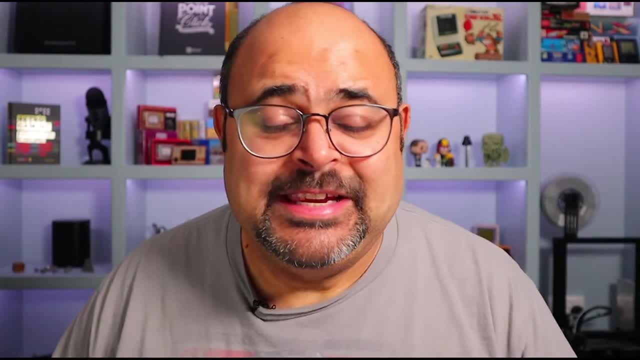 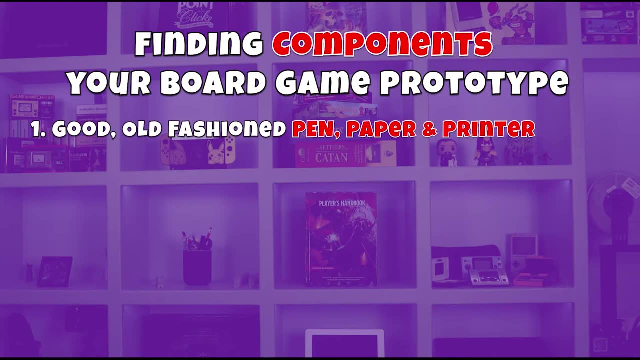 to build that little prototype. Well, here are six places you can find components for your first prototype. Number one: use pen, paper, cardboard and maybe a printer to create your components. That's what my son did to create his map tiles for his game. 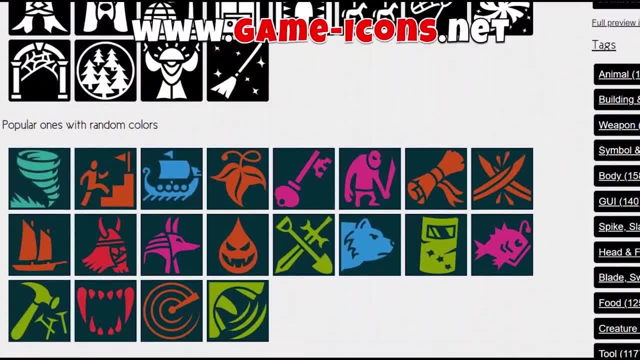 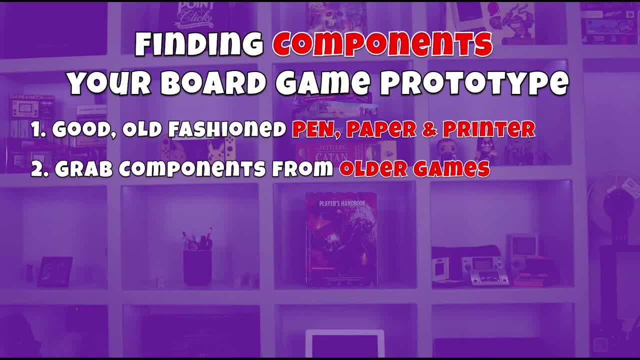 I, on the other hand, went along to gameiconsnet, printed out a bunch of icons and stuck them to some sticky labels to create my card game. Grab components from older board games or board games that you don't play very often, or even board games. 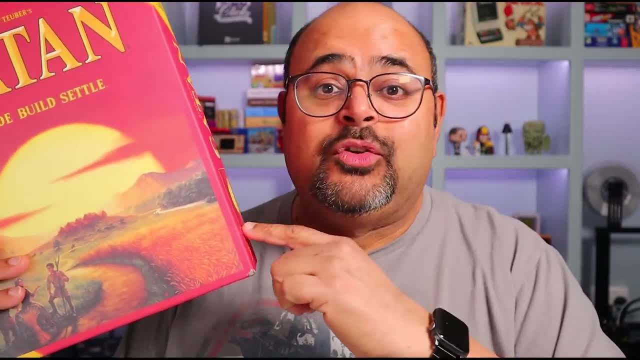 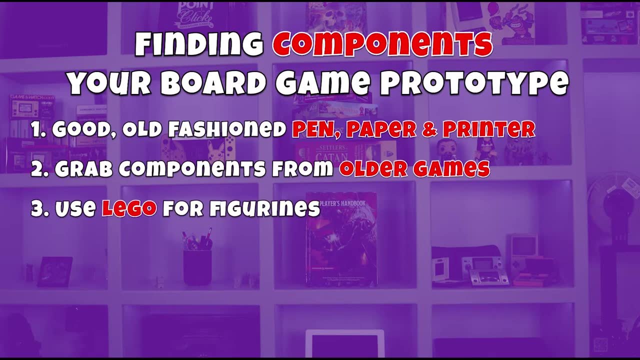 that you found in a thrift store, like I did with this one. This is a great source for picking up dice, as well as little meeples and cards. Lego, Lego is amazing and everyone's got some Lego lying around, As well as giving you little figurines. 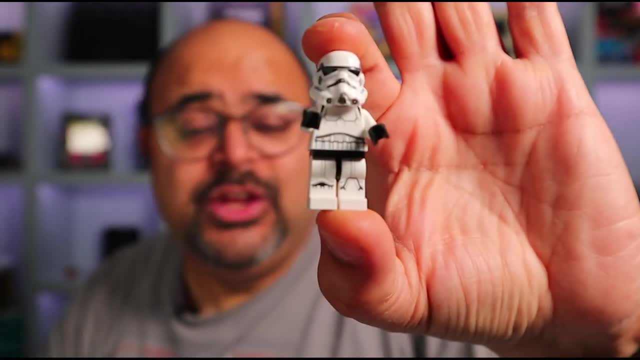 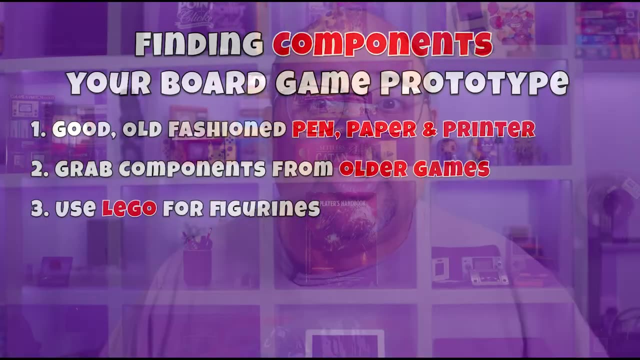 you can get all kinds of colored blocks, all of which are really useful in producing little components for your first prototype. Pop along to Amazon and pick up blank dice, blank playing cards- all kinds of things that you might find useful in building components. 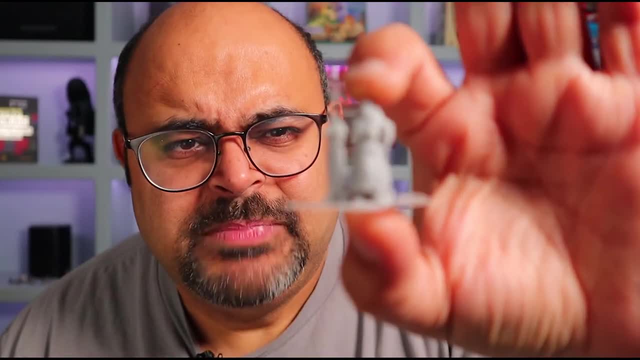 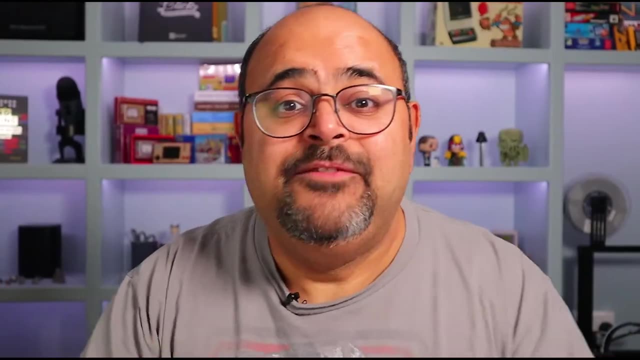 If you have access to a thrift store, a 3D printer, try printing your own. Just be realistic as to what you're going to achieve. That's terrible. And finally, if you want to keep your design process completely virtual, why not try Tabletopia? 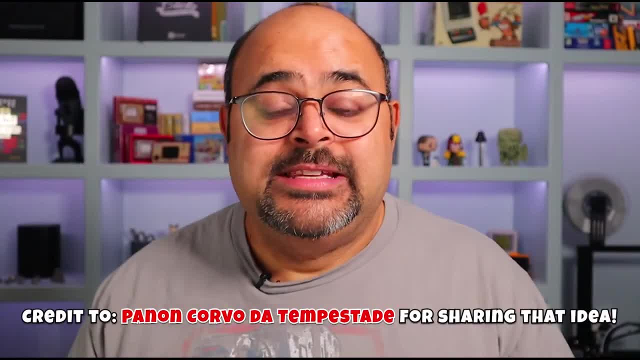 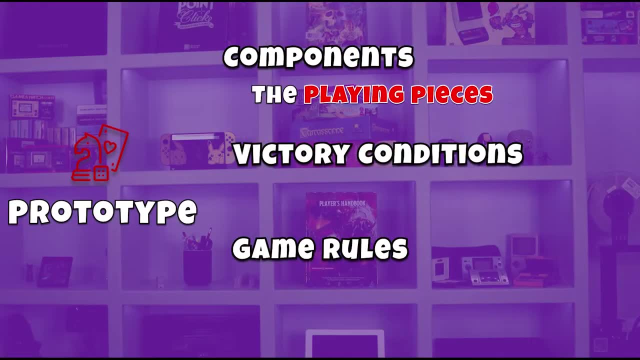 Here you can borrow from other components from existing games to help design your own. Okay, back to our prototype. We've talked about components, let's now move on to game rules and victory conditions. This will tell us how our game starts and ends. 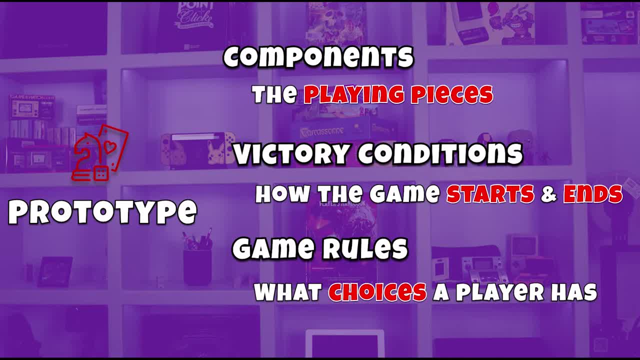 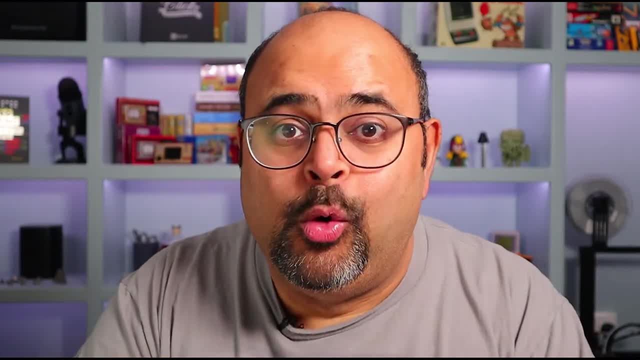 and also it provides a glimpse into what choices a player can make during gameplay. Allowing your players to make choices that affect the game and affect the end result is super important. in all good games. The rules will give you boundaries on what you can. 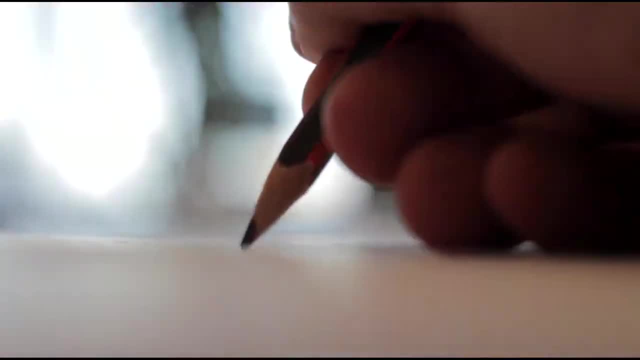 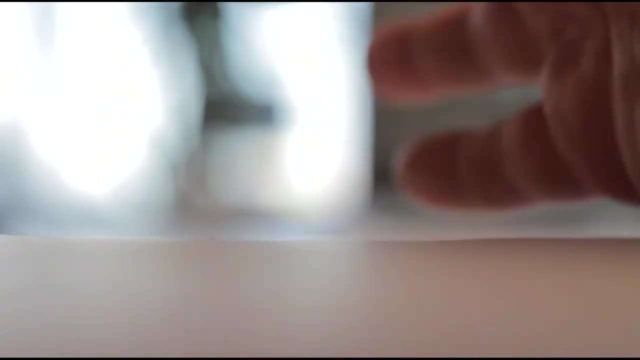 and can't do during your turn. But be warned, this is going to change often As you go through the process of game design, you're going to be visiting these rules and victory conditions over and over again and shaping them and changing them constantly. 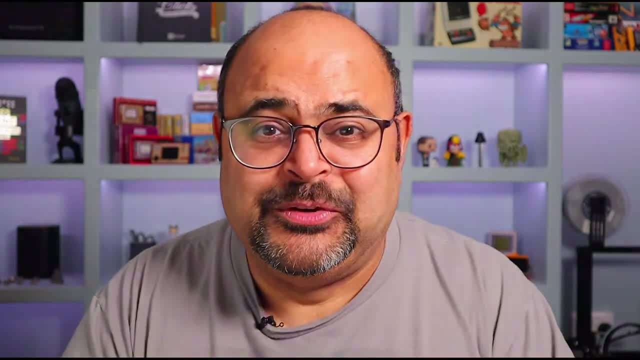 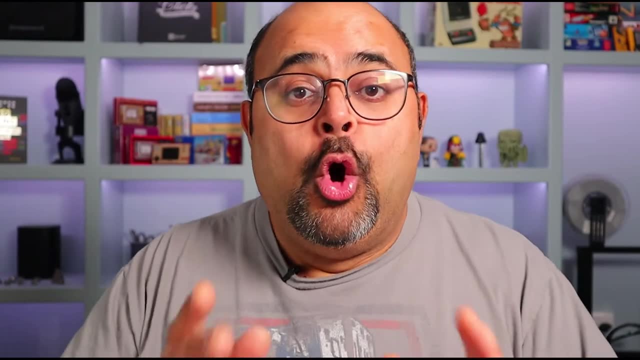 Don't get too caught up in this, because it's not going to be easy at this stage. Okay, so we've got a prototype. the next stage is to start testing it, or play testing it. Now you're going to start on your own. 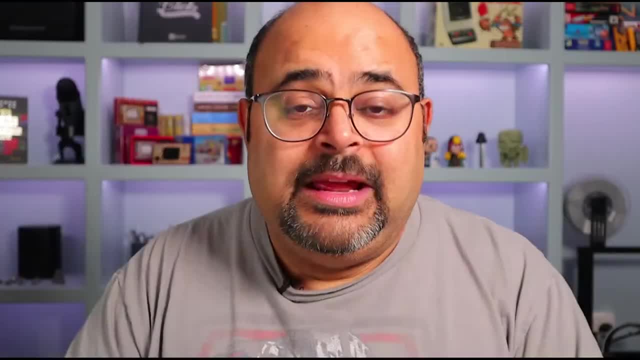 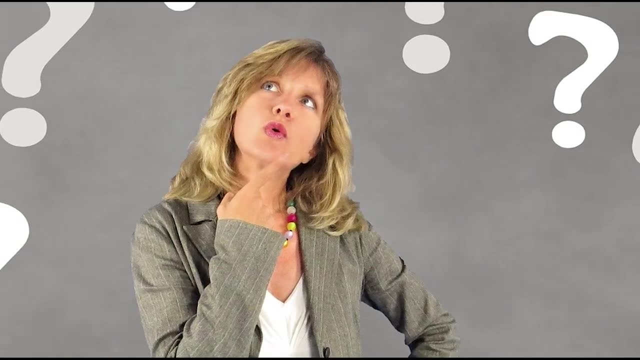 or with another creative collaborator, someone else who's helping you design the game. Now it's very important here to be harsh and brutally honest with yourself. Is this really the game you wanted, that you had an idea for? You've got to make sure you keep the theme. 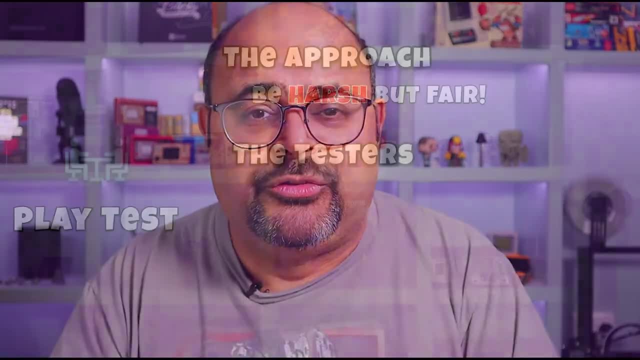 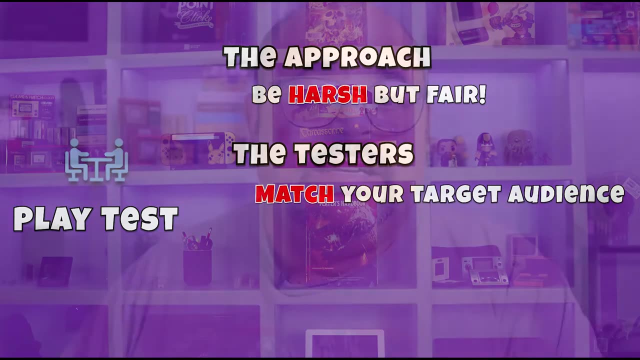 the player experience and, to some degree, the mechanics in check all the way through this process. A top tip here is to find a group of people to test your game that match your target audience, If you're building a kid's game that you just want to share in a classroom, for example. 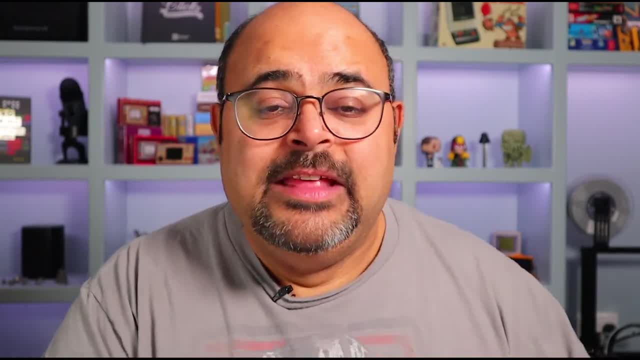 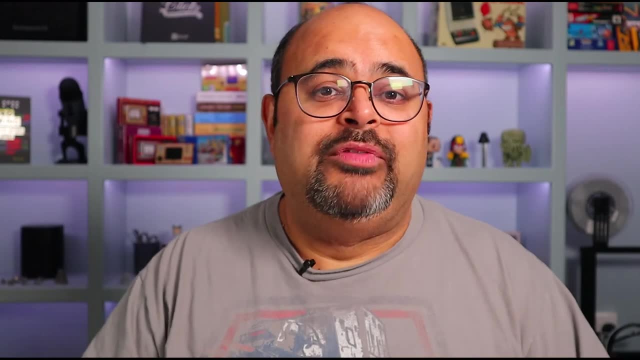 then testing it on adults probably isn't a very good idea. They're going to have a different response to the kids who are eventually going to play it. Now, when you first start testing, it's very likely that you're going to read the rules out loud. 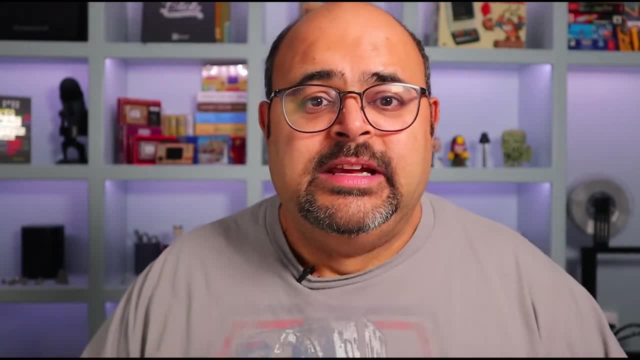 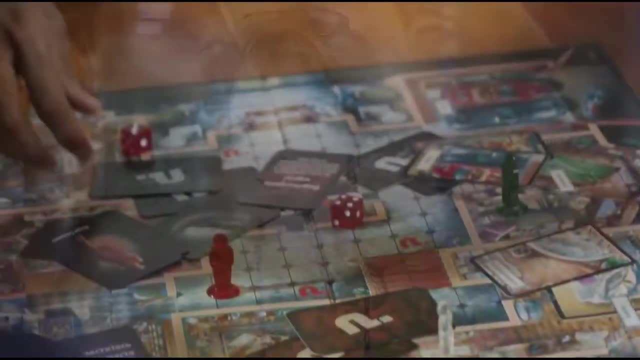 and, in fact, you may well be playing the game alongside your play testers, But as time progresses, you want to remove yourself from that position and just observe. What you're looking for are the reactions your players are engaging in when they play different aspects of your game. 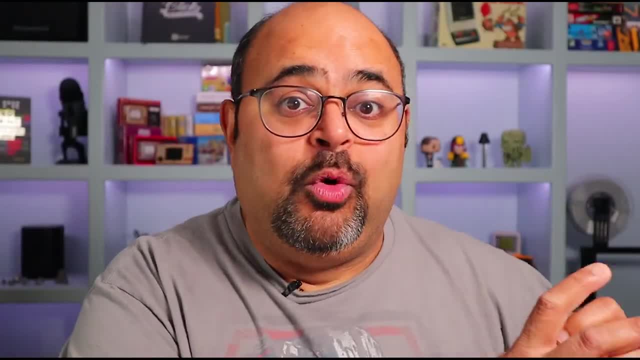 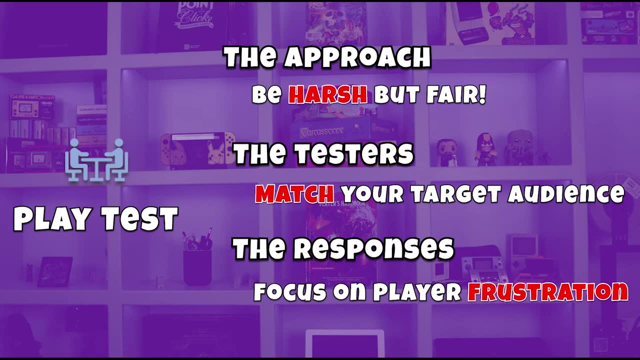 What are the reactions? Do they marry up with the player experience you wanted right at the beginning? What's really, really important here is to focus in on what frustrates your players. Don't listen to what they would suggest would improve the game. 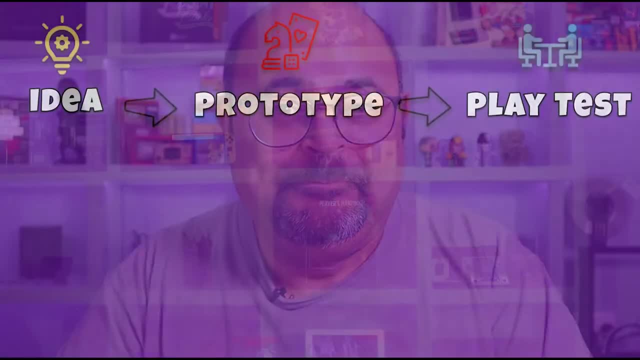 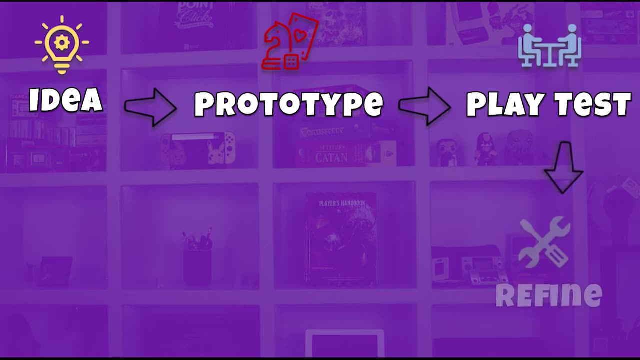 because, after all, you're the designer, not them. Now, this next step is an iterative step. That means it's going to happen over and over again. Each time you're going to refine and shape your game, You're going to take on board the feedback. 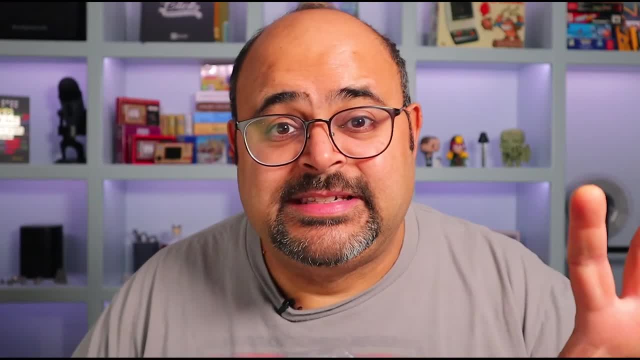 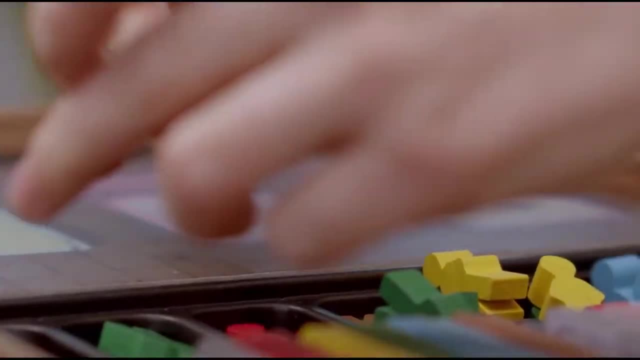 from your play testers. Now, remember, you don't have to listen to everything the play testers say, but very often what they say is significant, So you should at least record it. This is usually a really good place to look at what you can remove from your game. to simplify it: 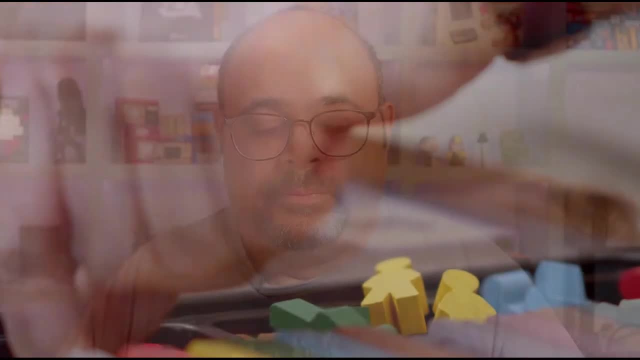 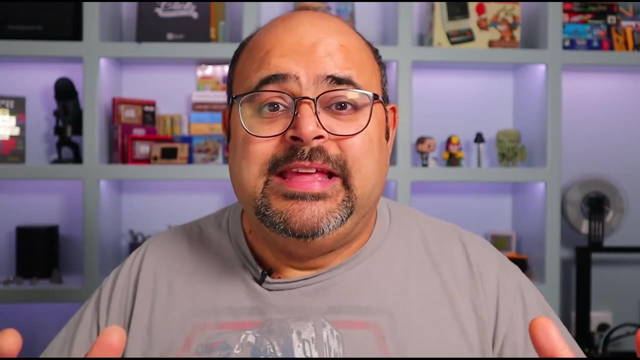 and perhaps keep some extra bits later as an expansion. To my mind, play testing and refining is actually the bulk of work when it comes to designing your game. You're going to be doing this potentially for months, if not years, for a really successful 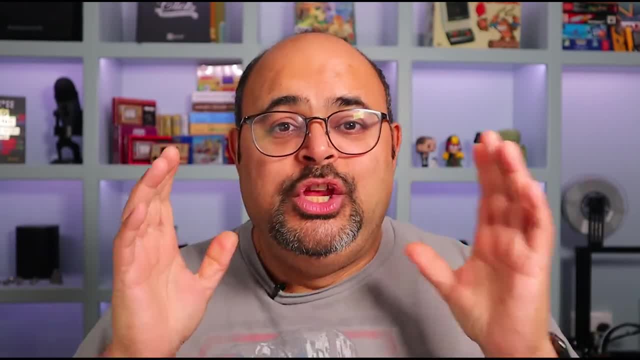 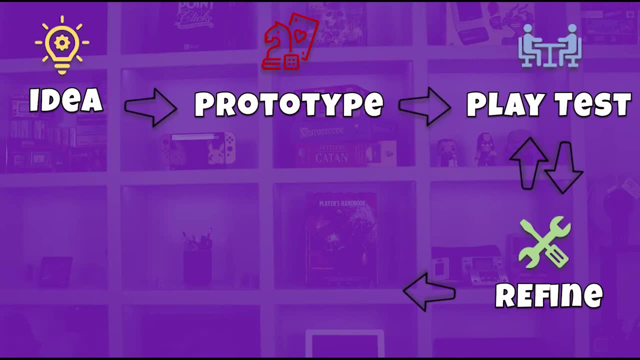 well-thought-out game. But that aside, once you and your play testers have both agreed that you've got the game as good as it can be, you've got your final product and you're ready to publish. Now publishing actually means a variety of different things. 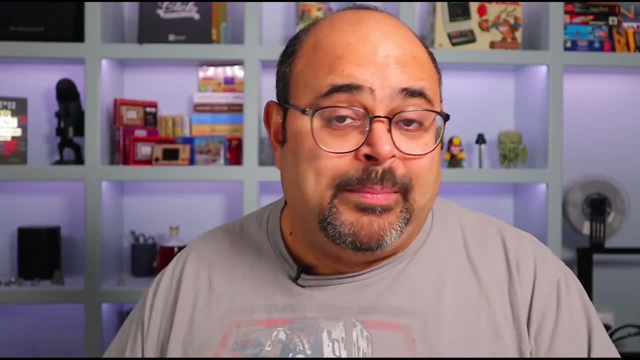 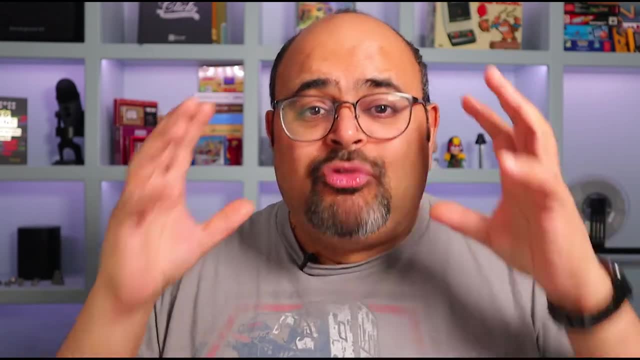 You may want to go down a formal route of finding a game publisher to publish your game. If that's the case, then just be aware you're going to have to probably give up a little bit of creative control. The great likelihood is that they have. 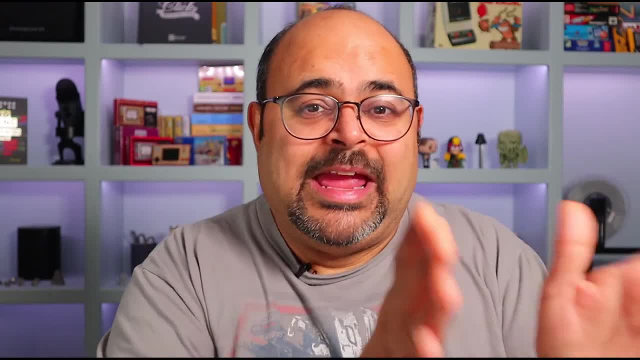 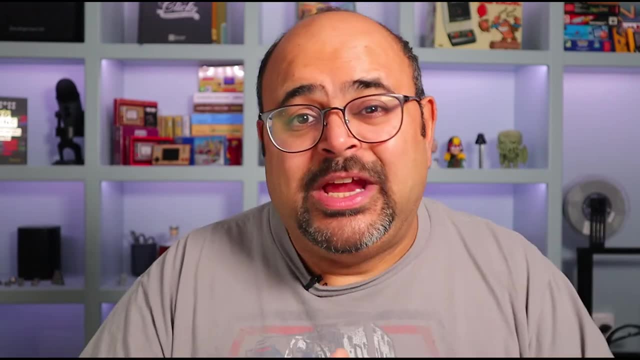 a particular target audience that they're going to want to position your game for. Now. that means that they will probably very likely in fact supply artwork and have their own artwork. They may change the theme slightly or even tweak some of the mechanics. 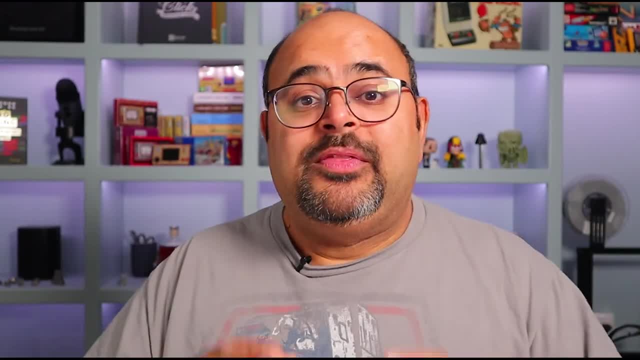 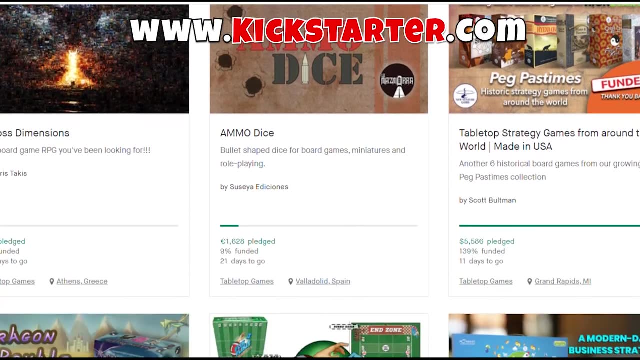 Now, if you don't want that, or if you decide you want to self-publish, well, this could be the start of your Kickstarter story. Here you're going to be doing a whole bunch of ad campaign and work before you actually get to Kickstarter. 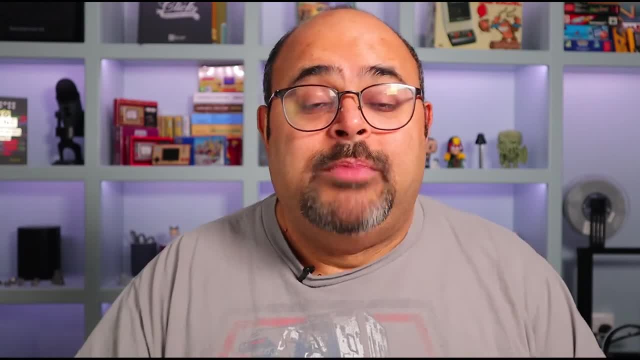 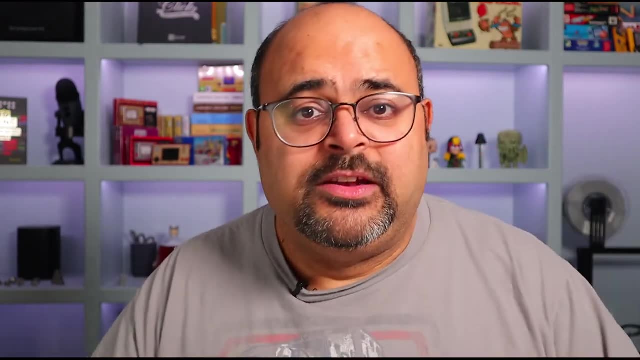 and that's a whole separate, different conversation. But one thing you need to do, probably, is find an artist, because what you've got so far probably won't be good enough. Find an artist who can actually spice up and make your game appealing visually. 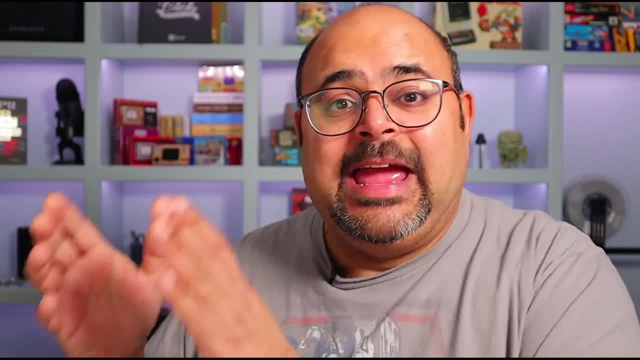 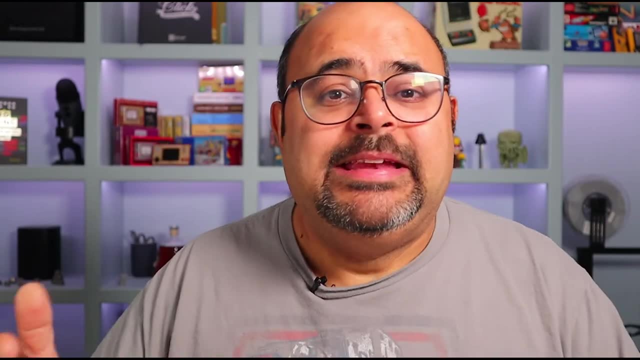 You're also, I would suggest, probably advised in getting a game rule writer as well, a professional guy to write your, or girl to write your rules. Finally, of course, you may decide that the game is just fine for you and your friends. 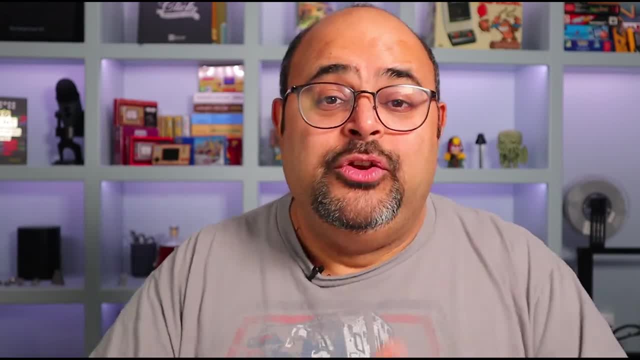 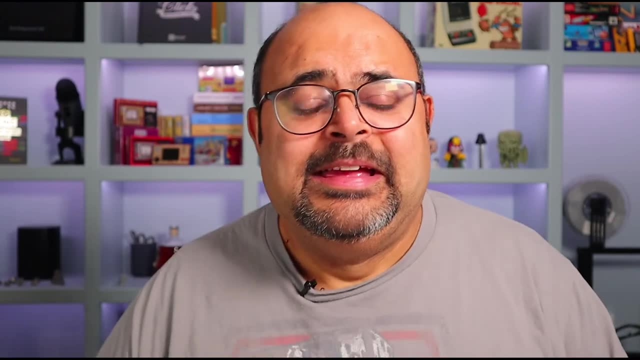 in which case, of course, the story could end right there. You can choose to spend more money in getting an artist and game rules written up and a box created, or you can stick it in a Ziploc bag and just enjoy it for what it is. 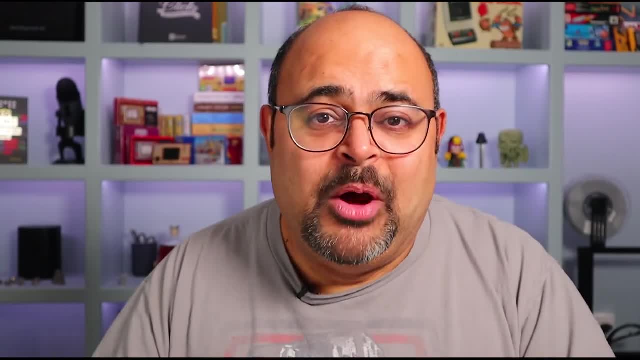 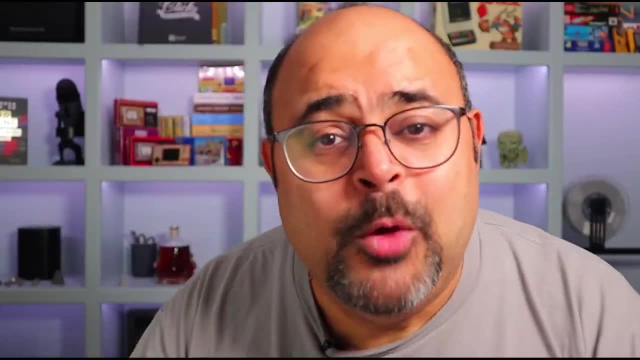 Either way, you can definitely now call yourself a bona fide game designer. Super duper, That's nice Way to go. Well, folks, that's my video. I hope you enjoyed it. I had a lot of fun making it. 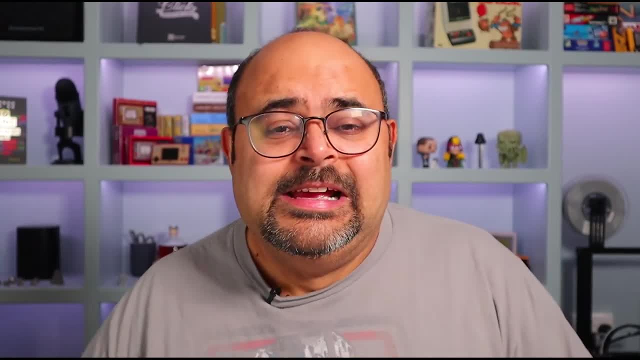 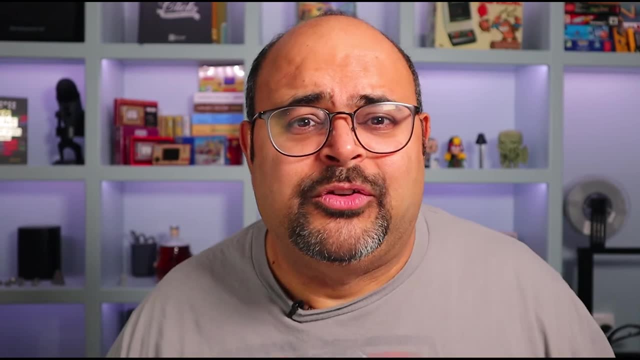 And recapping all the stuff I had learned in the last year. I hope I've captured it well. If I have, please do give me a like on this video, because it helps spread this video to others who may not have seen or heard of my channel. 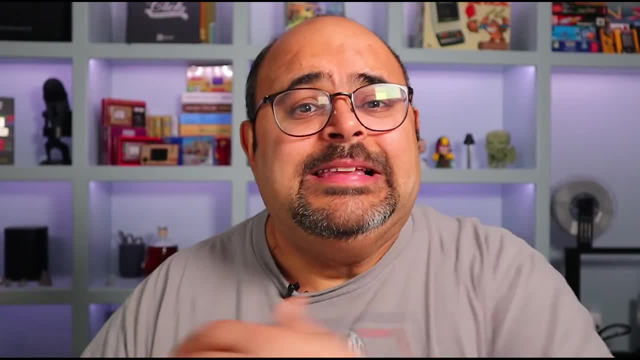 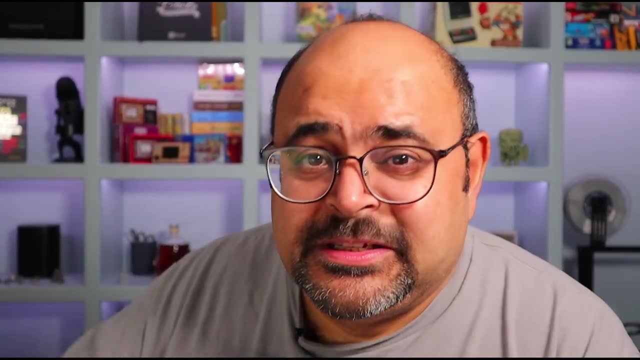 If I've messed anything up and if you think I've missed something, please let me know in the comments below, and I'll do my darndest to respond to each and every one of you. So until we meet again, folks, take care. 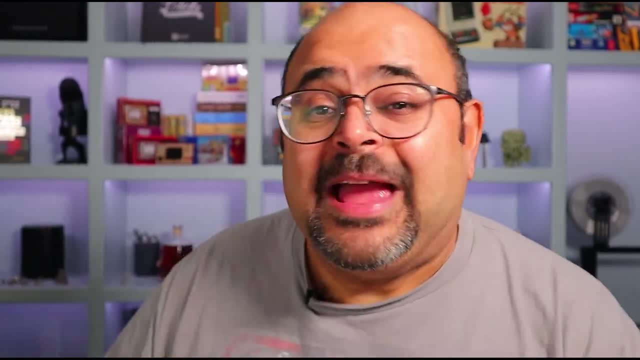 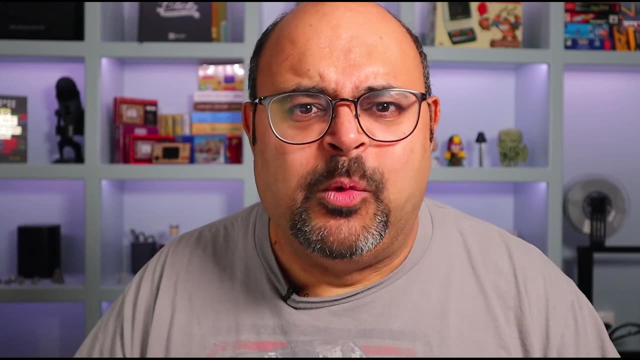 Oh, before I go, what do you think about the background music That was composed specially for this channel by my good friends Will and Lydia, Or Lydia and Will, depending on which way round it is. Anyway, I'm gonna put a description on the link below. and leave you with a little bit more of their music. 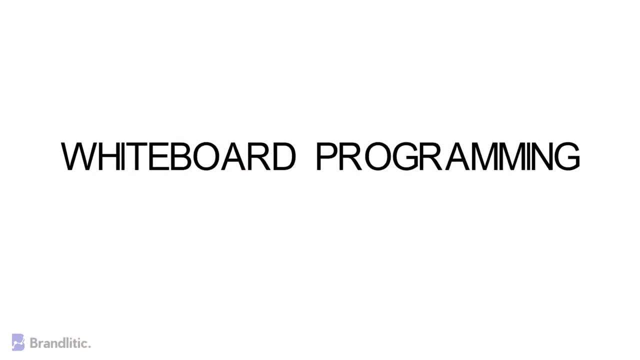 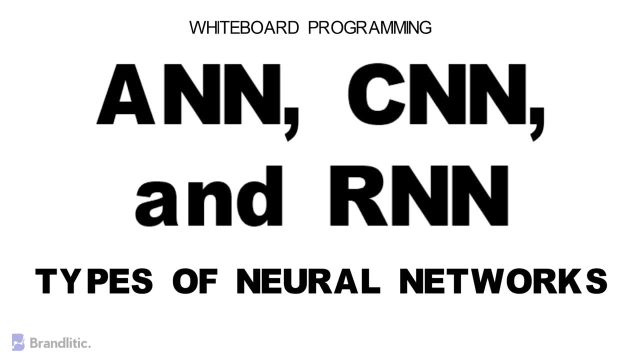 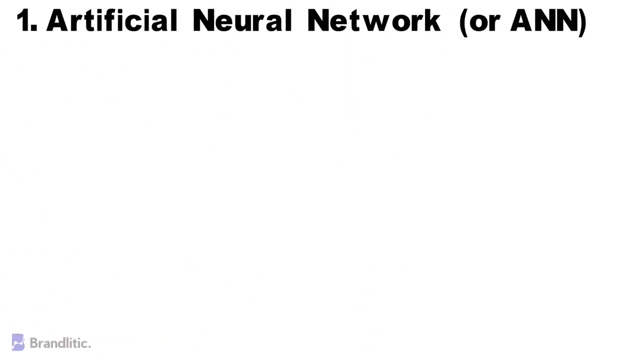 Welcome to whiteboard programming, where we simplify programming with easy to understand whiteboard videos. and today i'll be sharing with you the difference between types of neural networks or, to be specific, the difference between ann, cnn and rnn. so let's get started. first, one artificial neural network, or ann. well, it is a group where we have multiple perceptrons or neurons.